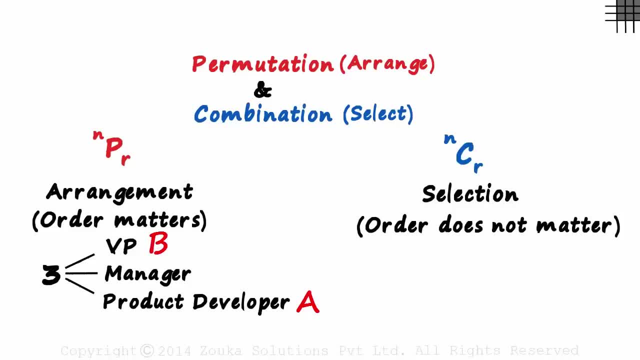 Or maybe A is chosen as a product developer, B as vice-president and C as a manager. Each case is different. On the other hand, if we are asked to select a leadership team of 3 out of 10 and told that it is a case of a combination, the order does not matter. 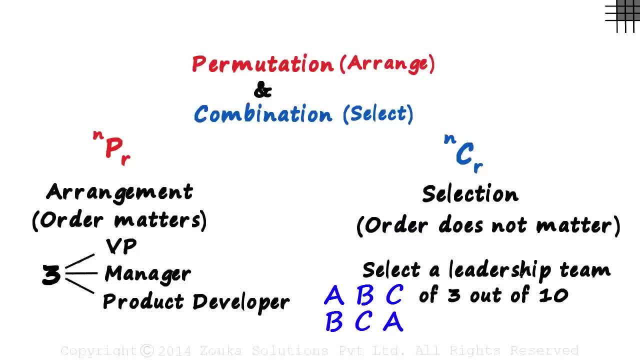 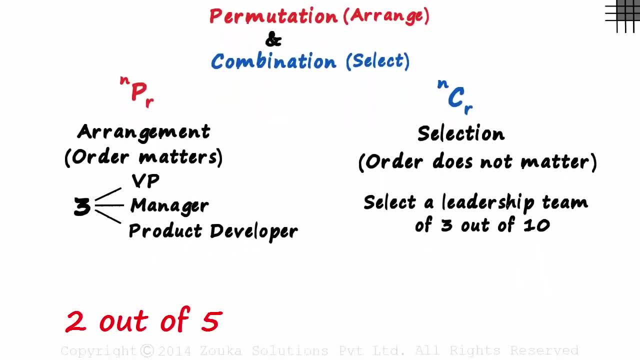 Selecting A, B and C is the same as selecting B, C and A or C, A and B. Take another example. Say 2 out of 5 people get ice cream, One gets vanilla and the other gets chocolate. This is a case of permutation, as each of the two people selected may get either vanilla, 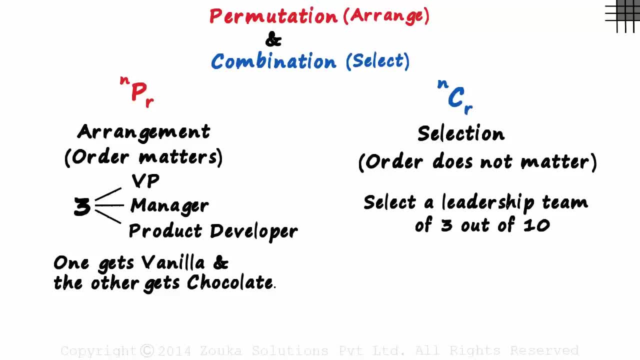 or chocolate flavoured ice cream, And if we adjust the order, then it is a case of combination. The order does not matter. If we are just told that 2 out of 5 get ice cream, it will be a case of combination. 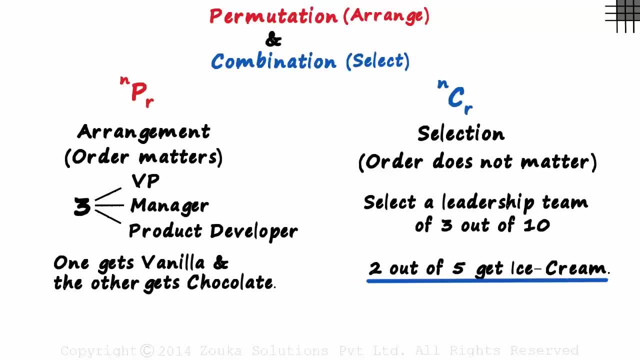 We aren't told anything else, Just that 2 out of 5 get ice cream. So the order clearly does not matter. Now that we have understood what permutations and combinations are, we can move on to the formulae. First we look at NPR. 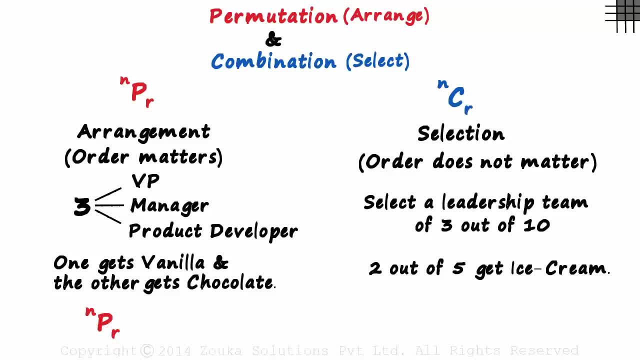 Arranging R things out of N distinct objects, and repetition is not allowed. For example, let's assume we have digits 1,, 2,, 3 and 4. And we have been asked the number of ways in which we can form 3 digit numbers using. 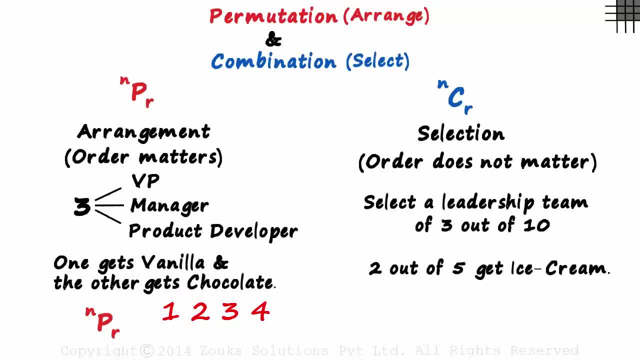 these 4 digits For this formula. we cannot consider cases such as 111 or 232 or 441.. The digits are repeated in each case, So the objects have to be distinct and there can be no repetition. So this equals N factorial divided by N minus R factorial. 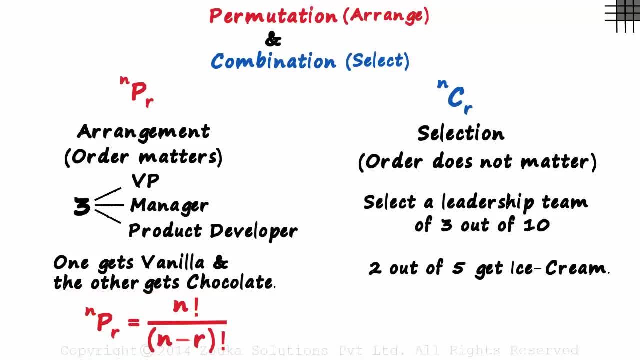 Yes, that's the formula. If we have to arrange 3 people out of 10, it will equal 10 factorial divided by 10 minus 3 factorial. Don't worry, we will look at numerical examples later. For now, let's just look at the formulae.